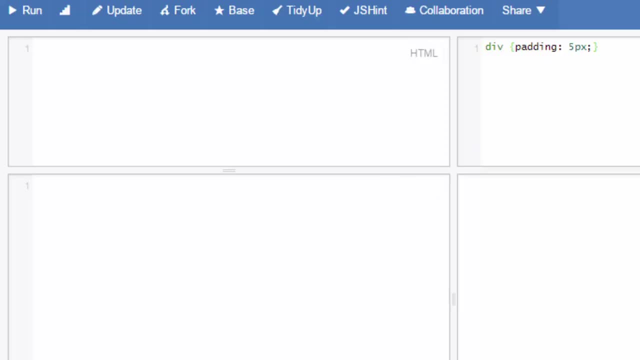 to attempt to drive home some of the things we've learned in previous videos and also demonstrate the power of custom directives and why you would use them and make it hopefully very easy to understand. Okay, so a lot of people who are just learning Angular get to custom directives and they 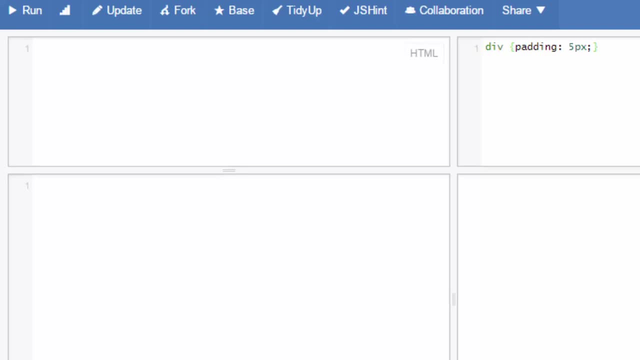 ask: well, why are we doing this when the same thing could be accomplished in a simpler way? And let's do an example of what we're talking about. So in some previous instances we're using ng-repeat to output some results. So we might. 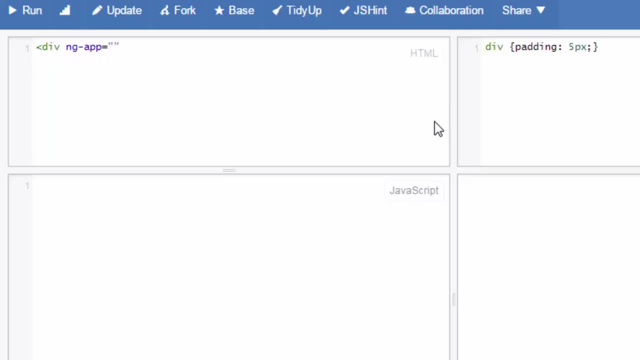 have something like this with an app. Let's say again that we're building the user list. We'll call this ng-repeat And inside of this, like we've done before, we'll have a controller And we'll call this user list controller. And what we're going to do here is we're going to just loop through. 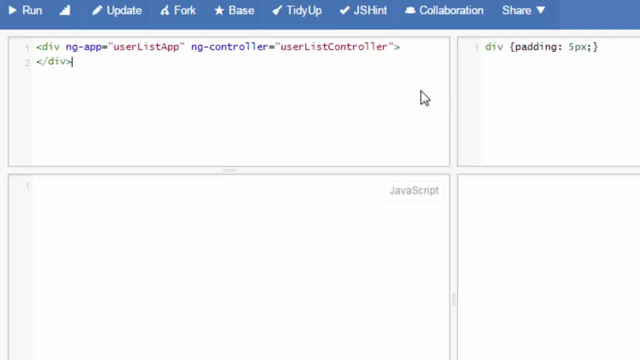 a list of users and output them to the screen. So in previous examples, what we did is we did, let's say, a div tag with ng-repeat on that, And we'll do u in users. So each user will result in a div tag being output, And 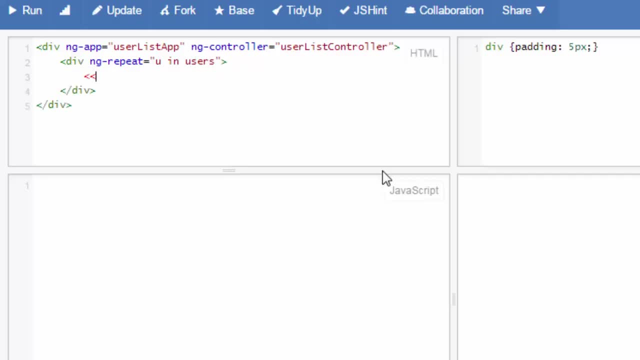 then inside of that we might have put something like name And we'll start with email. So let's go down here then and implement the actual app. So we'll have our user list app. Find that as a module And then, in our controller, is where we will actually want to bind that. 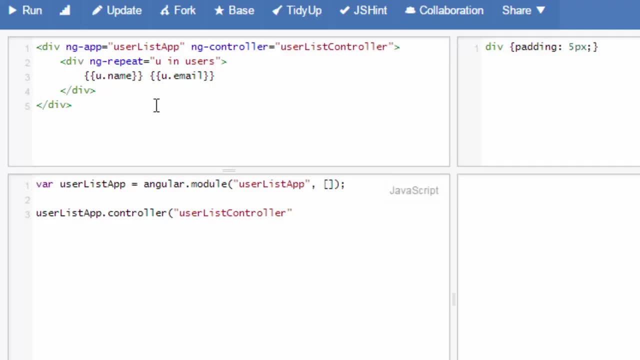 collection of users in so that we can access it in this ng-repeat statement up here. So we'll use Angular scope and HTTP variables, just so things fit nicely on one line. This is only for readability purposes, Okay, And then we'll call HTTP. get on our list of users. 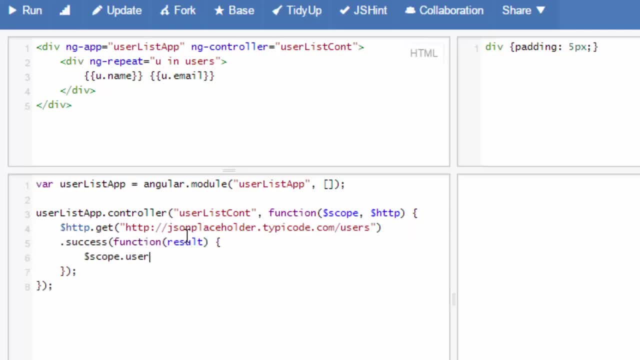 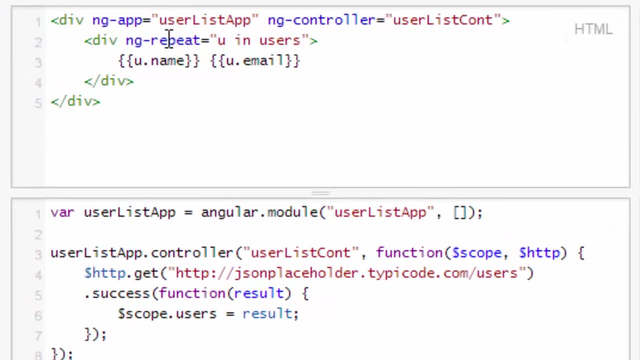 And, on success, we'll bind the result to our users. Okay, When we run this, we get a list of users. Now, let's say we're interested in formatting. So one way we could do that is by putting the HTML tags around each of these user properties right here. So we'll 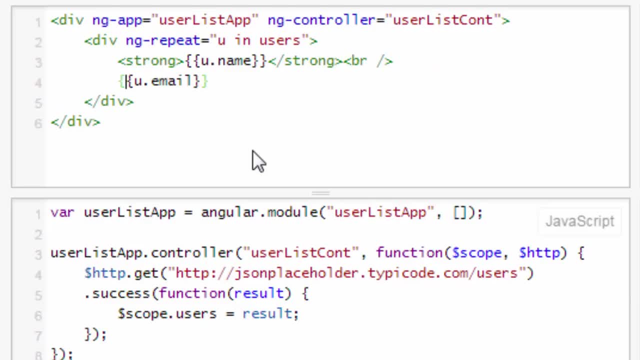 bold the name And under that we'll have the email address And we'll also add in make this a user roster, So we'll add in phone number And finally we'll add in their website as well And we'll put that inside of an anchor tag so their website will show up and be clickable. 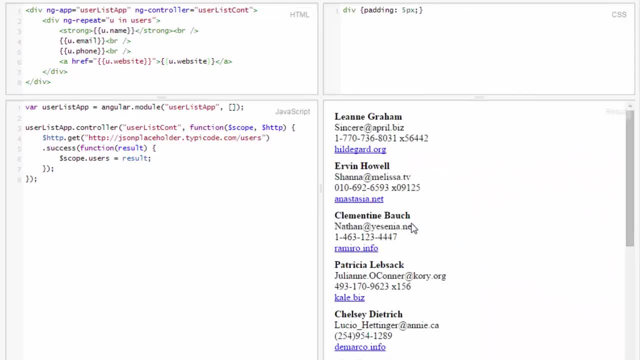 Okay, So there we go. We get a formatted list of users. This is very basic, But now there, we've done some formatting. Okay, So now let's say that we want to display a specific user elsewhere on our page, maybe at the top, in the same format. 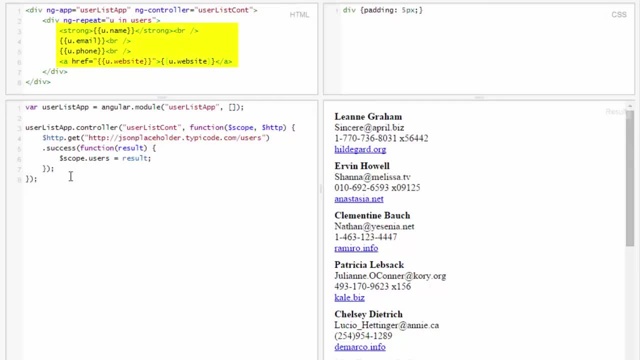 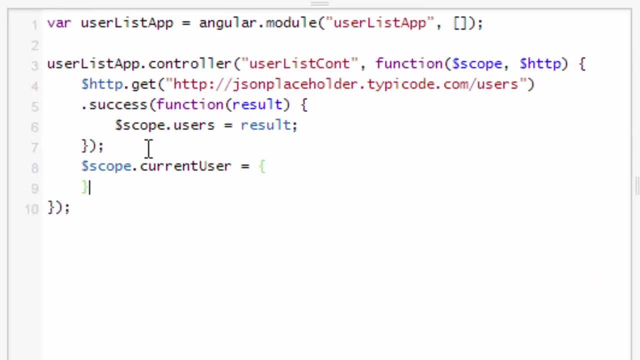 Well, using this pattern up here, what we would have to do is define a new user. We'll call it CurrentUser, And we're just making this up. We could call it whatever we want to really, And we'll give this. I'll fill in my own contact information here. 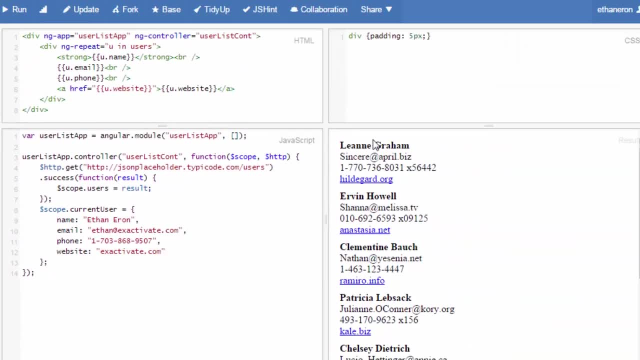 So I've got this current user object and I want to display it at the top here and have it be highlighted in gray. Let's just pretend we're building an application that highlights the current user. So, using this design pattern, what I would actually have to do is duplicate this HTML. 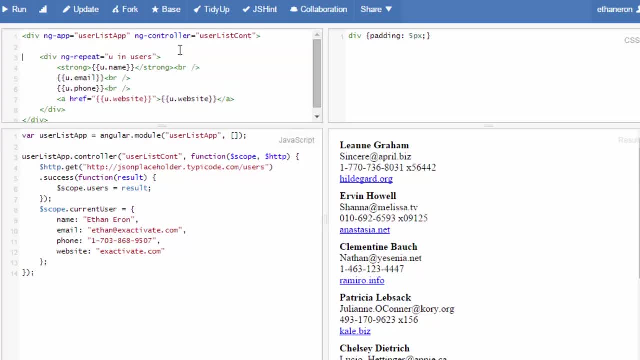 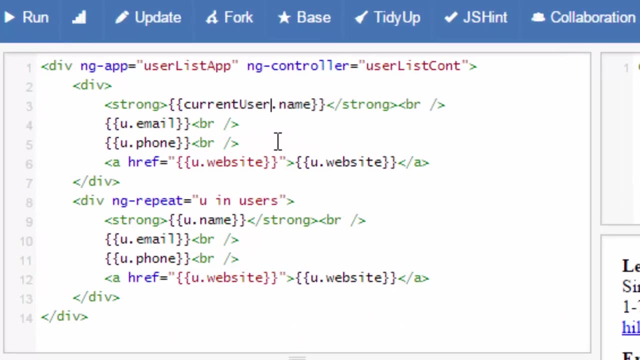 content right here. I'd also have to probably put it inside a div tag to get the necessary padding around it. So then I would have the HTML duplicated here like this, and I would also have to remember to call current user and just shorten it to current, just to make typing a little bit easier. 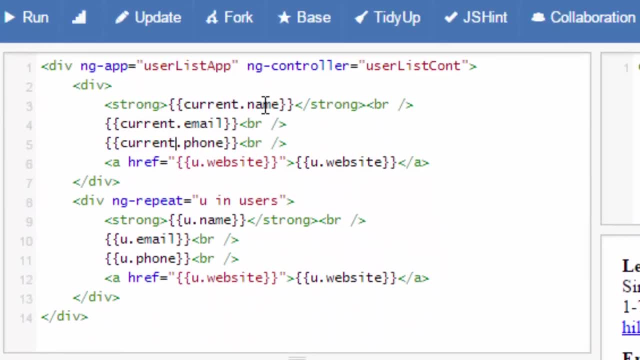 So we'll call it current And we have to replace every invocation where U has been used with current, because we're actually using current. The current user is DIDO And we'll call it new because it's a different type of stuff. 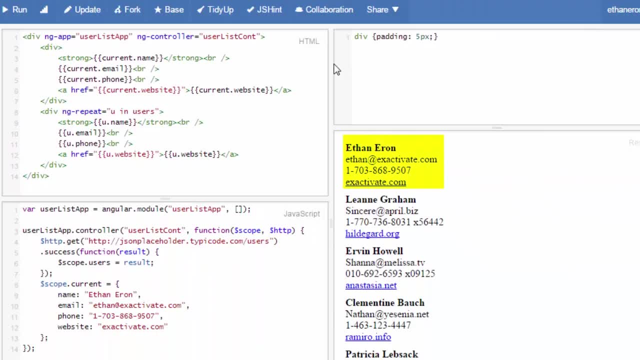 Let's call it highlight. And now also remember we've got to duplicate all of this code, So we're going to have to duplicate this code here. This isn't a big deal. for a simple example, In the code file we just have to duplicate it and bring it to the state of the file. 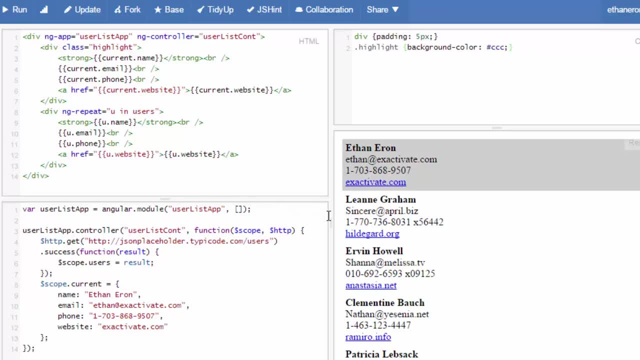 So we don't have to put something in there that of course might have like a lot of like color in there And we'll just leave that. So we're going to have to duplicate that And let's see what we can do. simple example, but, as you can imagine, for a more complex application you might want a way to share. 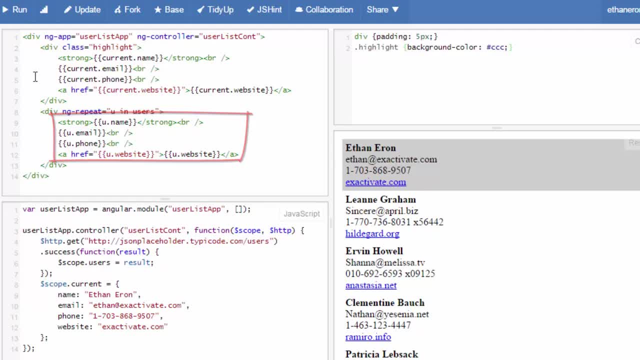 this display without having to write the same code twice, Because imagine if each of these were displaying 50 fields or 100 fields- which wouldn't be unreasonable- This could become quite unwieldy. One way we can accomplish that is through using a custom directive. So the way we do that is: let's 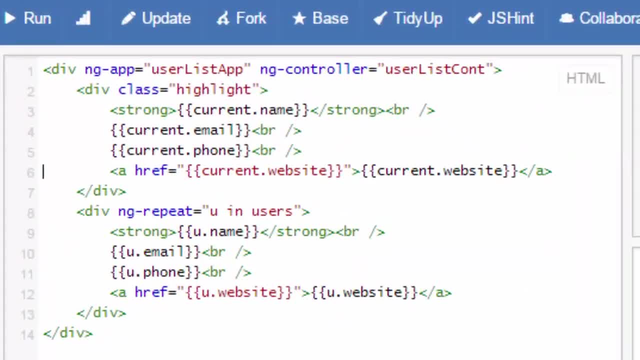 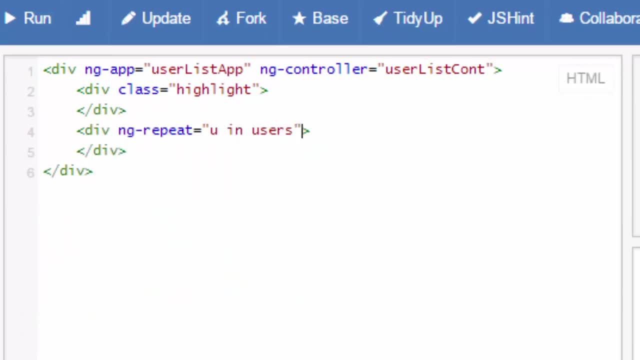 call our directive custom user. So I'm going to eliminate this stuff right here and this too, And I'm going to make this tag have a directive that I'm going to call ng custom user. And actually this is a good time to also say that, as a general rule, when creating custom directives, you should 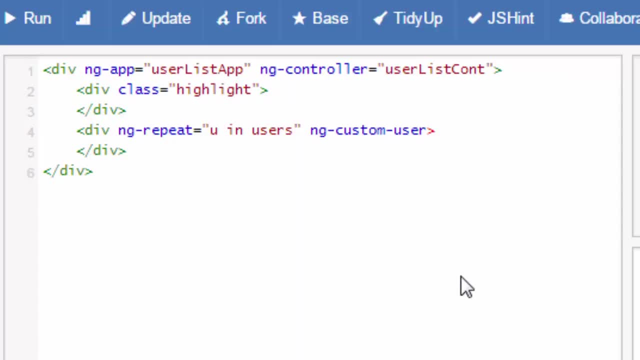 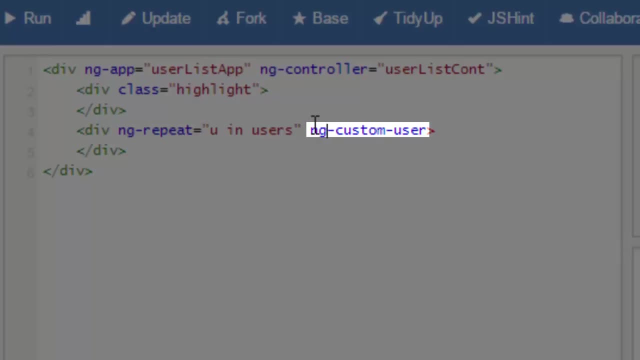 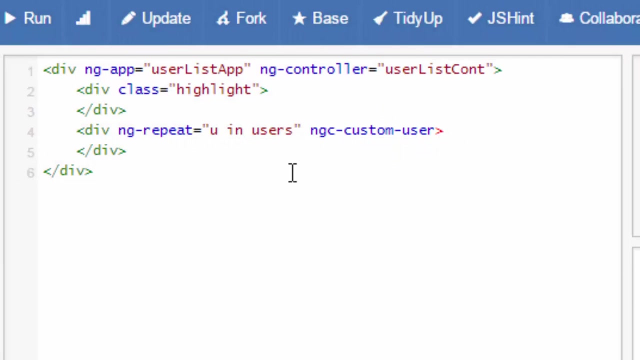 use a different prefix besides ng because in the future Angular may end up using this name right here to implement A native directive in Angular. So if we go ng c where c stands for custom, it's unlikely there would ever be a future collision with Angular using that. So from now on we'll prefix any custom directives. 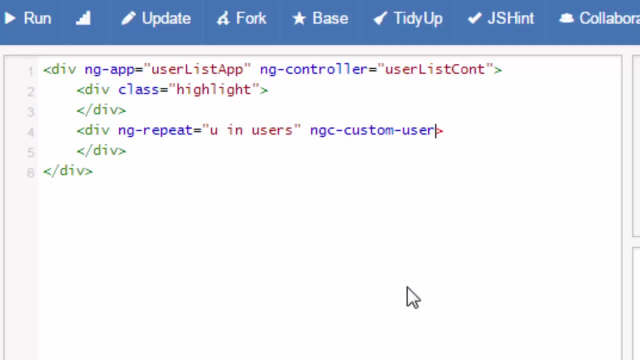 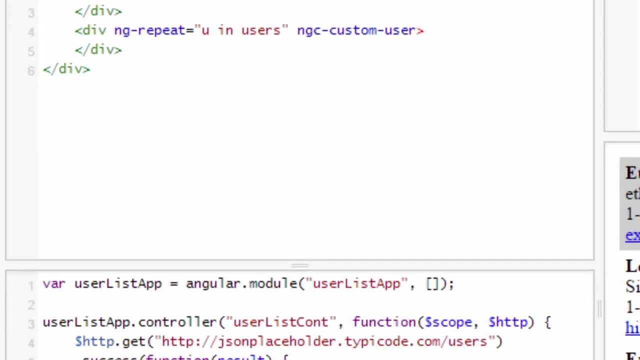 as ng, c and then the name of the directive. So now we've got our custom directive, but we also want to be able to process whichever user is the current one in this loop. that's occurring right here in Angular. So let's set up the directive first. Use the directive call And remember we're calling that ng custom. 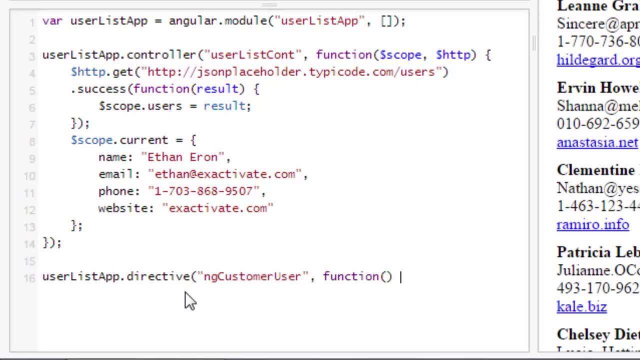 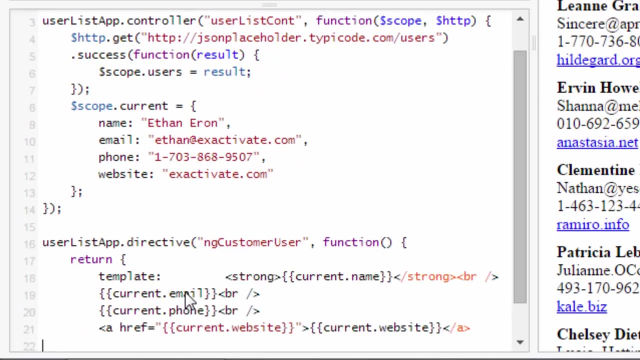 user And we'll get that function, And then inside, we will be returning what is basically our directive object. Okay, so the first thing we're going to do is use what is called a template, which we've seen before, to format the user who's being processed. 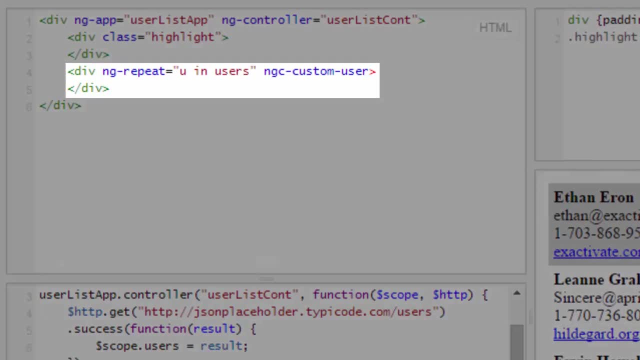 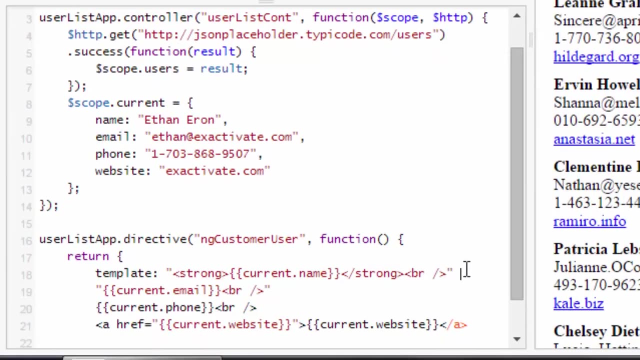 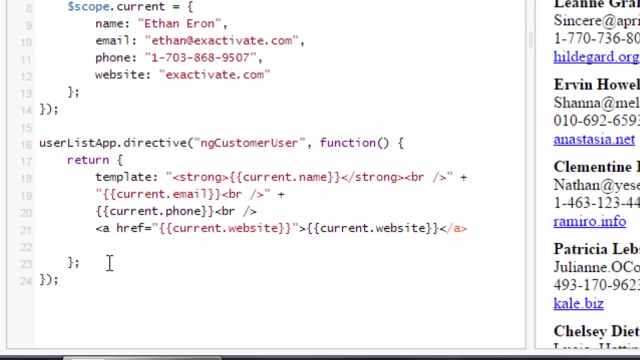 So whoever the current row is up here in this ng-repeat, we will process a separate instance of this directive for that. Now, for longer templates, you can load them from a separate file. For this example, just to keep it readable. we're going to put all of the code in here, like so. But if you had a very complicated 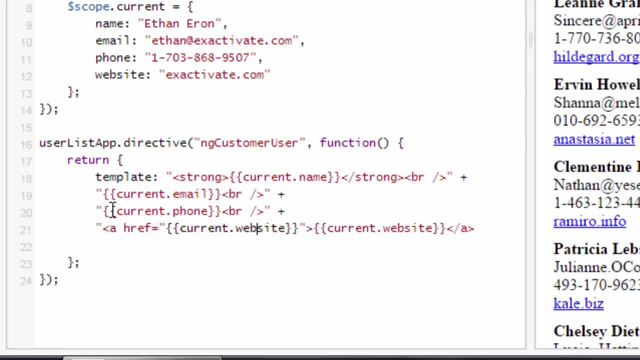 template, there's no reason why you couldn't load it from its own separate HTML file. Okay, so there's our template. I just have to escape these double quotes right here. Okay, Now, unfortunately, if we try to run it like this with, let's say, we changed it to uname, So if we tried to run it like this: 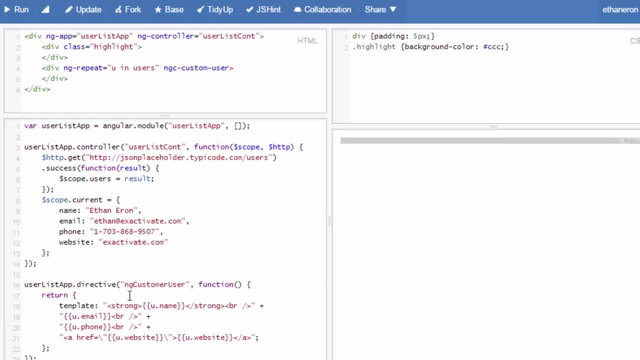 nothing happens. It doesn't know anything about who this user is, And there's a variety of reasons for that that have to do with scoping. So what we can do is arrange to pass in this current user right here, So 亸, And we can pass it in with whatever argument name we wish to use. 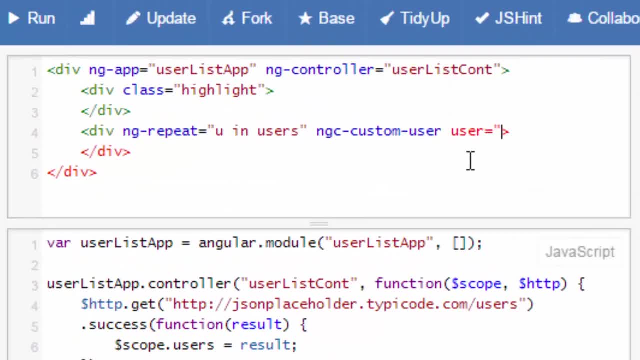 So let's say we want to just be able to specify the user. We could say: user equals you. We could also call this person, call it whatever we want, call it MGC user. Let's just call it user for right now. 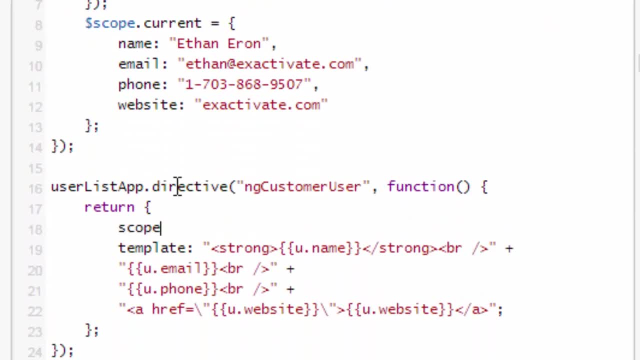 So now, when we want to read in this user object, we can do so by giving this a variable name that matches whatever we used in the template, in this case you. And then we want to read in the argument up here, on line four: 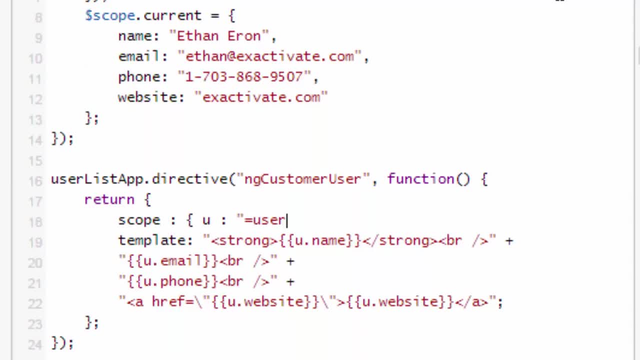 And the way we do that is by saying equals user, which tells Angular to read in the entire user object. If we were passing in just a string, like just the user's first name or email address or something, then we would use a different syntax. here. we'll use an ampersand and we'll 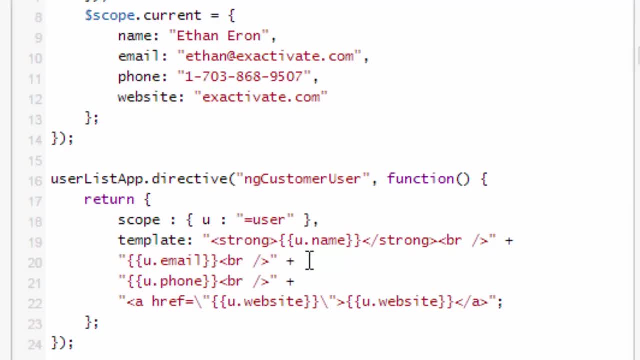 show it. We'll show how that works. But for reading an entire object in, we go equals. and then the argument name to match the name up here on line four. Number two: make sure your directive name matches. Now those two names match. 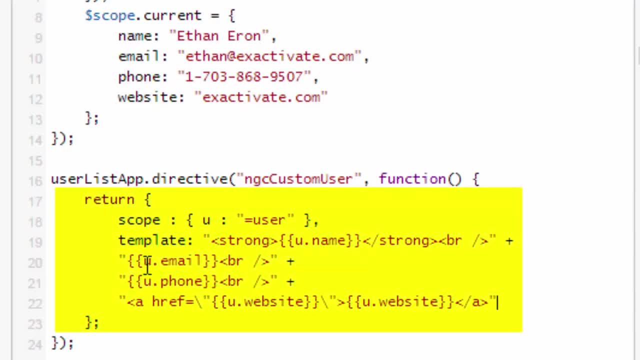 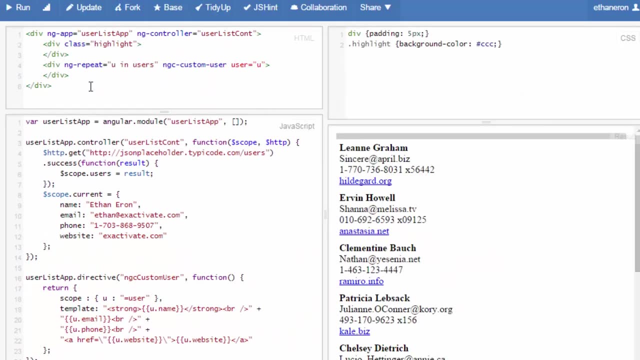 And there's also an extra semicolon down here. This is an object literal, so you do not want to use semicolons inside of an object literal like that. So there it is. Each user has been passed in and formatted according to this. 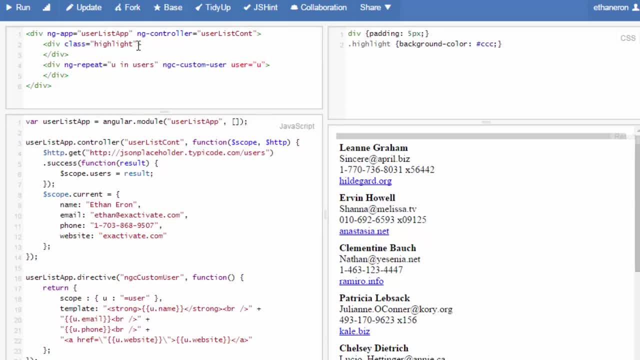 So we're going to do this template pretty nice. Now for the highlighted user up here, we could do the same thing. We use the ngc custom user tag And for the user we'll give it scope: current user, which we defined right here on lines. 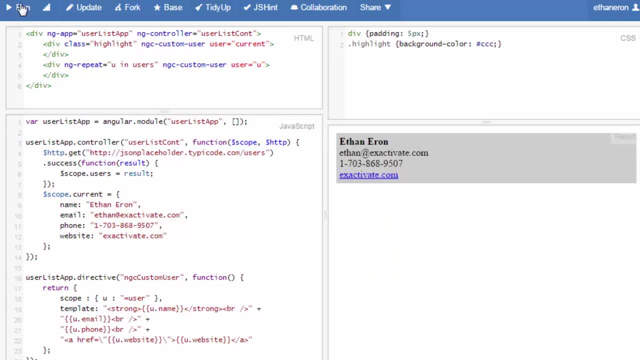 eight to 13.. So now we should get a highlighted user at the top of the page, followed by the remaining users. We only have to create this template code here once and we can use it throughout our application to style items. So we can use it for items like this, which is handy. 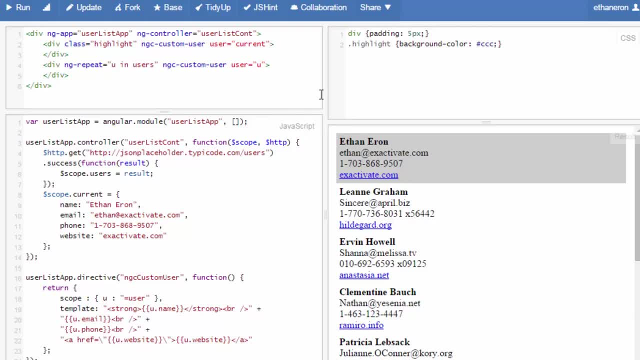 We also mentioned about being able to pass in labels that were not objects such as text. So let's say that we wanted to provide a label. We could call this caption, We could call it whatever we want. Let's call it label and LBL for short, just to show. 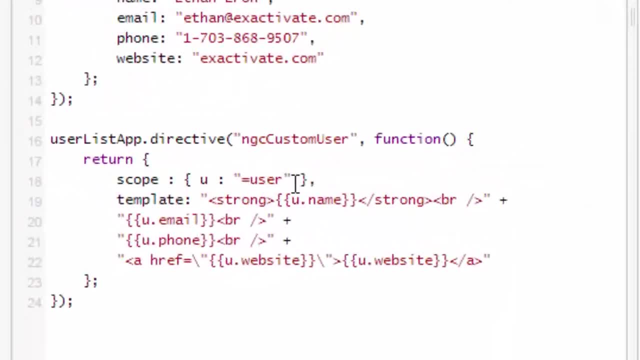 And we want to be able to specify that as an argument. Well, we can easily add that to our template here by first providing a scope Variable, which we'll call L for short, and we'll read that in as a string. So, unlike here, where we're reading end user as an object, we're reading in label as a. 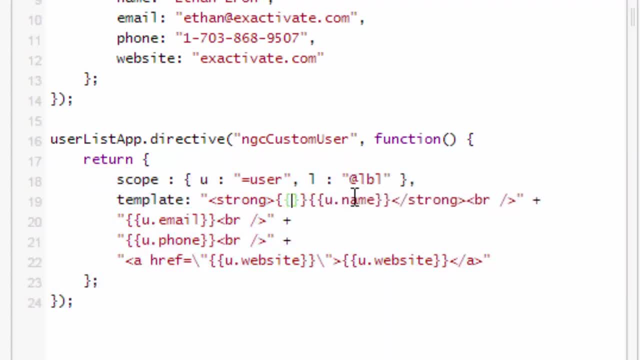 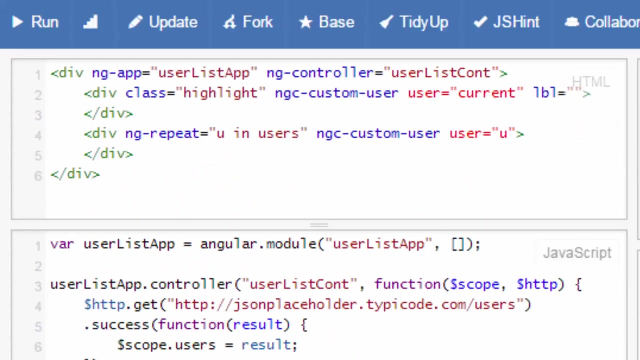 string. We can then include the label in our template, calling L, not LBL. It follows whatever we use here. So our label- this is only this- is all native to the template and it will add that label to our template. Let's say we want to put our current user, we want to have an asterisk next to our current. 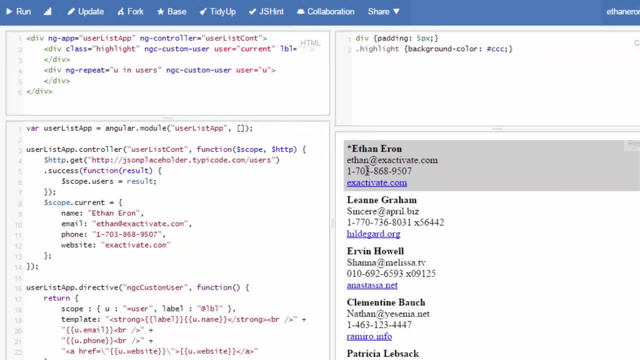 user. So we put the asterisk And it shows up next to our current user but not next to any of the other ones, because we've just specified it here. There's obviously a lot more that we can do with custom directives, but this course has. 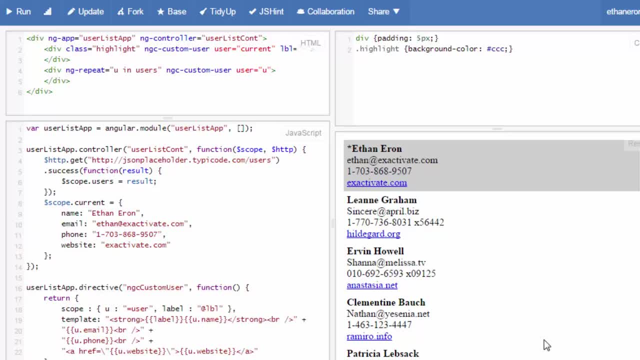 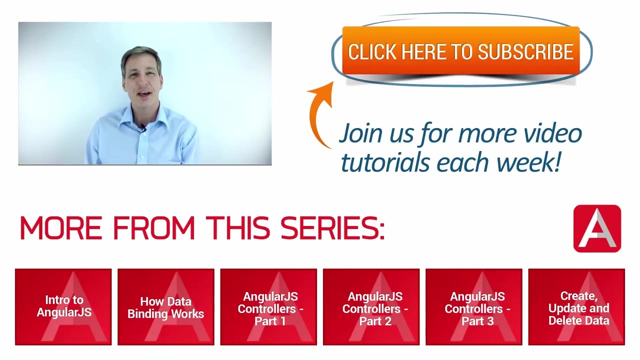 given us a good intro to that and other Angular concepts and allows you to see the different powerful features that are available. All right, Thank you very much for watching and happy programming.